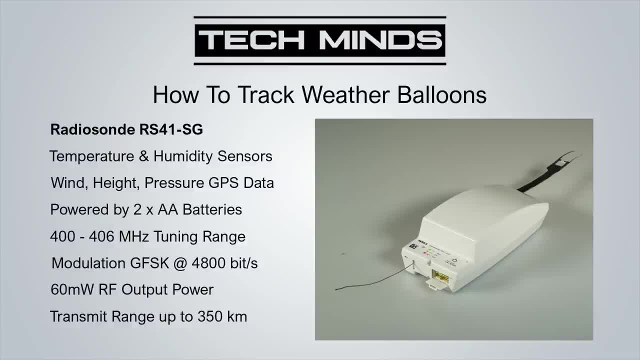 radio sonde. Now this contains a dedicated sensor for temperature and humidity. Other data can also be transmitted back to earth, such as wind speed, height and pressure, but this information comes from an onboard gps receiver. Now the whole thing is powered by two AA batteries, which provides just 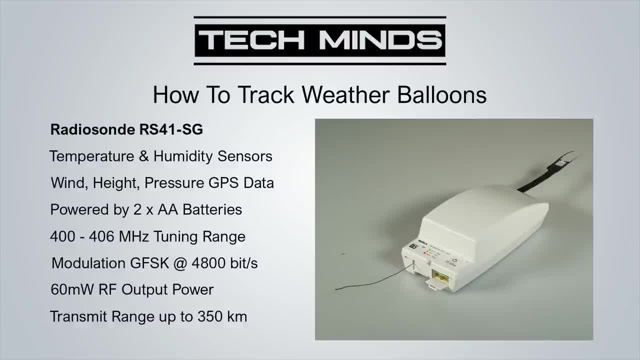 three volts. Each radio sonde can be programmed with a different frequency so that if you have many launches taking place at the same time in the same area, you can alter the frequency that it transmits on anywhere between 400 and brand new. So if you have a radio sonde that transmits on 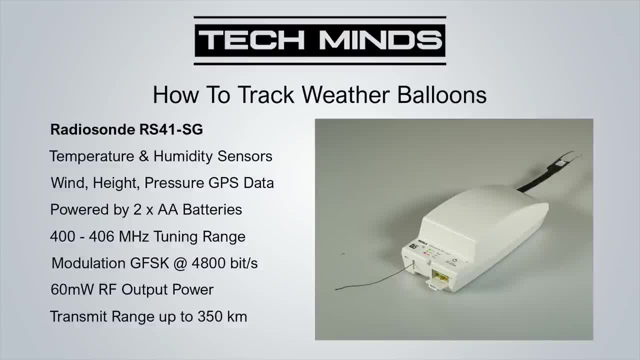 406 megahertz. Now, the modulation type being transmitted from the RS-41SG is GFSK at 4800 bits a second, and the maximum output power is around 60 milliwatts. Now, 60 milliwatts doesn't sound like a lot of power, but when you are 25 miles above the earth, that 60 milliwatts will. 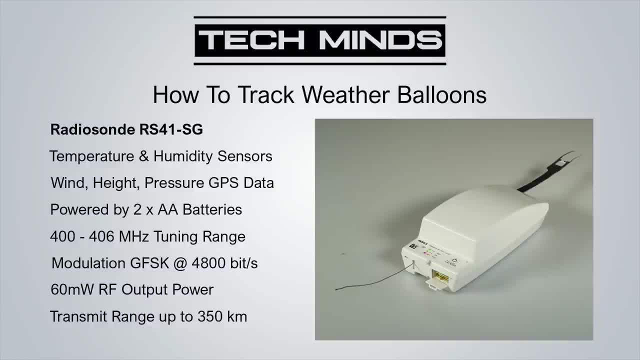 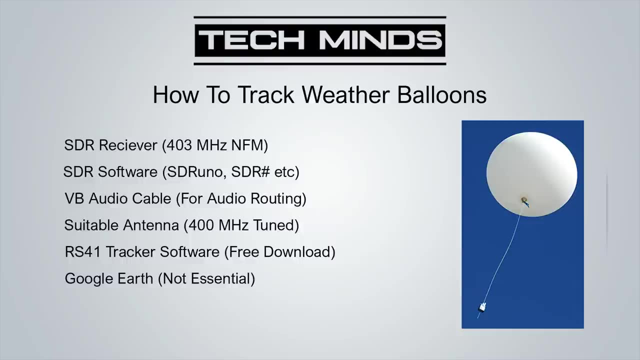 cover a wide area. In fact, the RS-41's predicted transmit range is actually around 350 kilometers. So to be able to receive and decode these transmissions we will need some software and hardware. So firstly we'll need an SDR receiver that is capable of receiving narrow FM at around 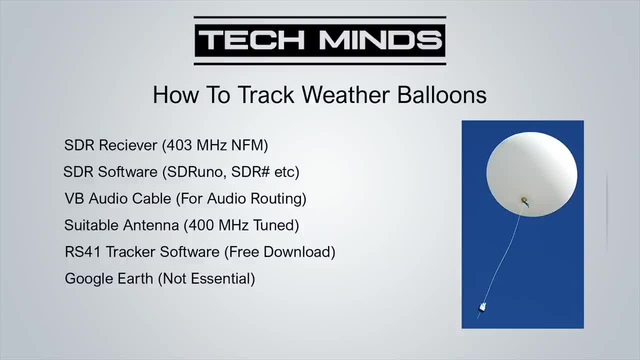 403 megahertz or between 400 and 406 megahertz. We will then need our SDR software, where we can then use VB audio cable to route the audio to our decoder. You'll also need a suitable antenna. The antenna that I'm using in this video is just my dual band co-linear, which covers two. 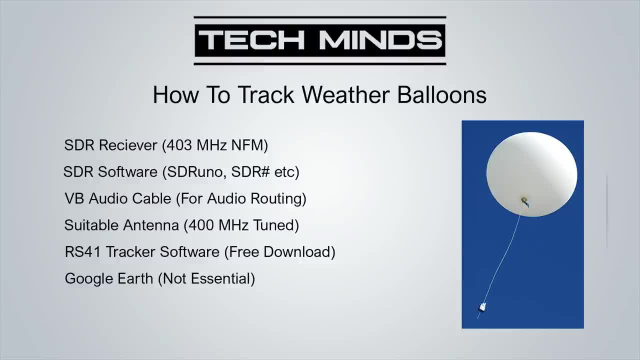 meters and 70 centimeters. The 70 centimeters band is from 430 to 440 megahertz, so even my antenna is not strictly tuned for 400 megahertz. Another possibility with regards to which antenna to use could be the use of a small Yagi antenna pointed towards the balloon. Now the decoder software also. 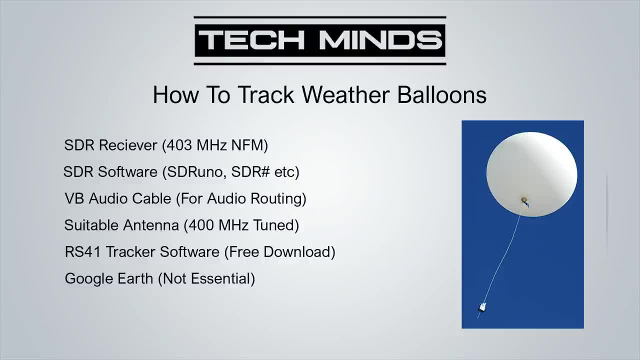 has the ability to control a rotator, so a Yagi type antenna can be kept pointing at the balloon for the duration of the flying. The software for decoding these transmissions is called RS-41SG. The software is called RS-41 tracker and thankfully the author has made the software a free download. 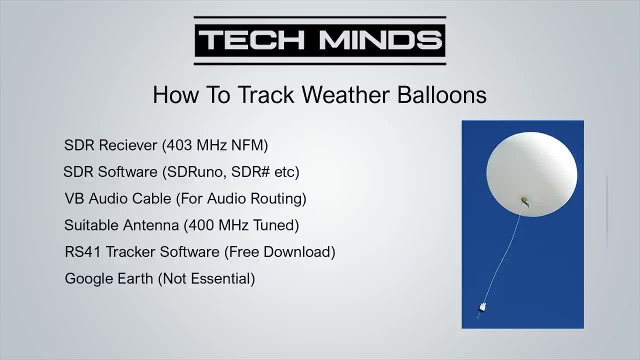 although it is encouraged to drop them a donation, if you like, and use their software Now. there are other software packages which can perform a similar task, such as Sond Monitor, but for this video I'll be showing RS-41 tracker. I'll leave a link down in the description of. 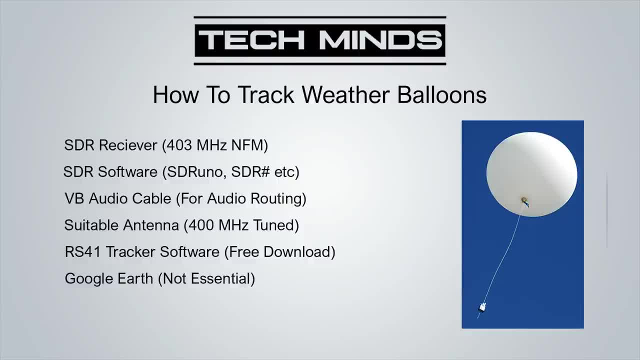 where you can download this from Now. an optional extra is Google Earth. I'll show you why you might want to install Google Earth a bit later in this video. So the SDR receiver that I'm using is called an RS-41 tracker I'm using. this video is an RS-PDX from SDR Play. I'm also going to be using SDR Uno. 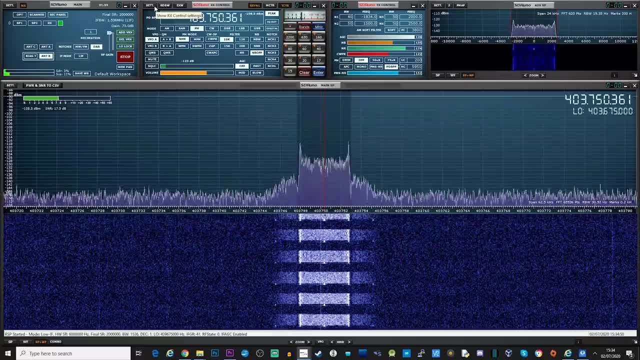 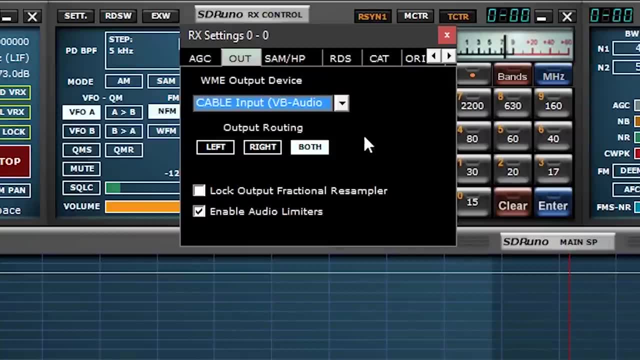 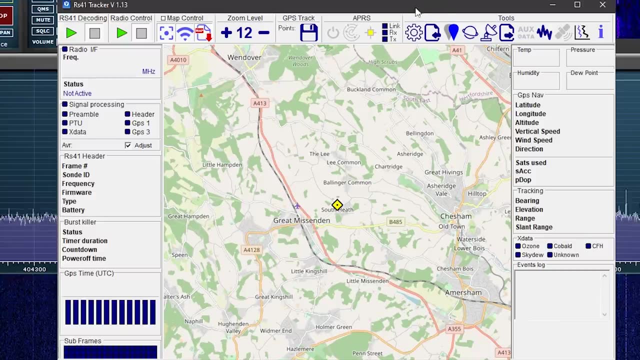 for the receiving software. After we have VB audio cable installed, we need to set the SDR software's audio output and point it to VB audio cable. We can then go ahead and download RS-41 tracker and start the application. Now there are two items that we must configure before we can start using. 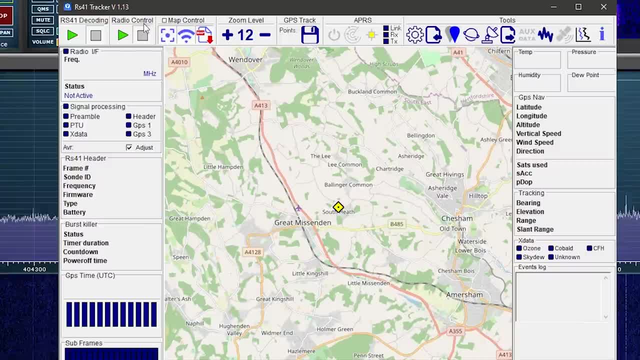 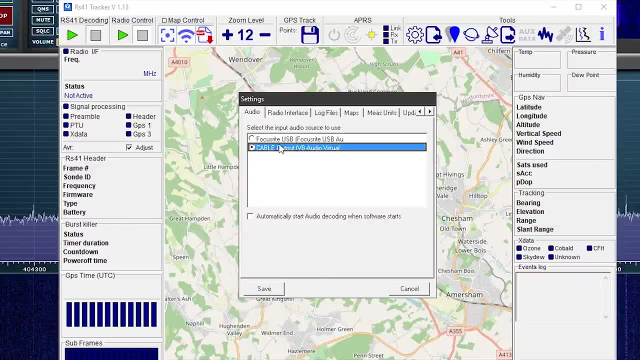 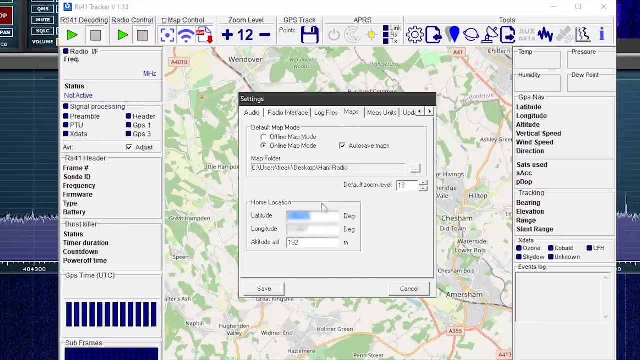 the software. The first item to configure is where RS-41 tracker takes his audio input from. In this case we'll be setting it to VB audio cable so that we get SDR Uno's audio piped into RS-41 tracker. So the other setting we need to edit is the home location. Now this can be found under the maps tab. 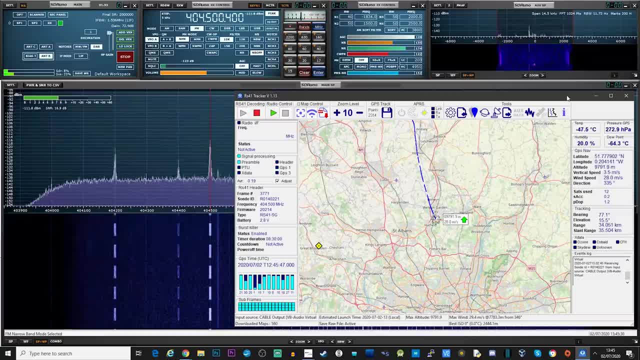 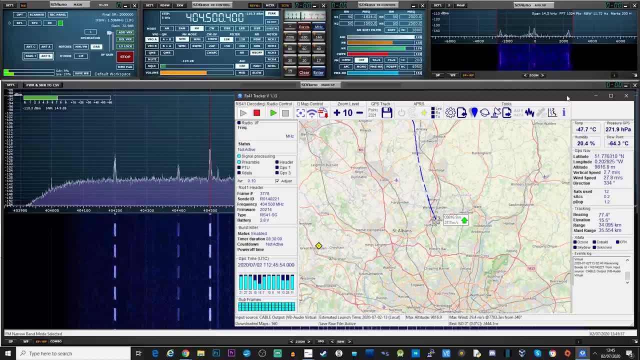 within settings. Go ahead and into your latitude and longitude for your location. This information helps RS-41 tracker present you with the data relating to the balloon's bearing elevation and range from your location. This also helps when you're using a rotator with a Yagi antenna. 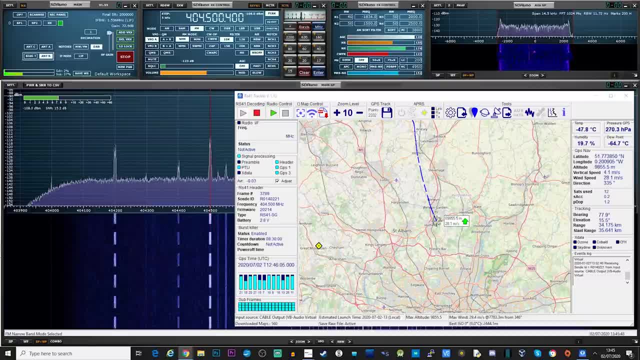 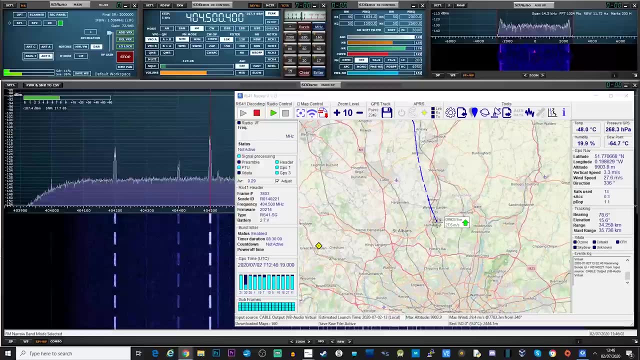 Once you've found a radio sonde transmission, set the modulation to NFM and the bandwidth to around 4 kilohertz. You can then press the green play button on the top left of RS-41 tracker to start the software decoding the balloon transmissions. As you can see here, we are now successfully. 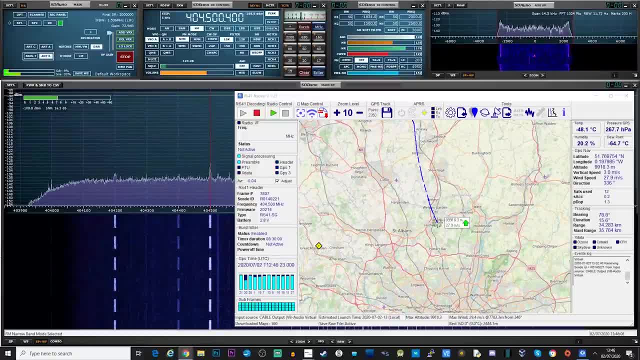 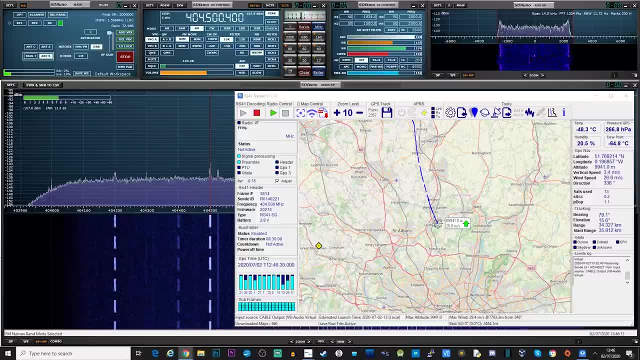 decoding an RS-41 SG transmission and RS-41 tracker is displaying its location on a map, And there's lots of other bits of information on this screen. Let's take a quick look at each of these. So first off, on the top left, we have the signal processing. 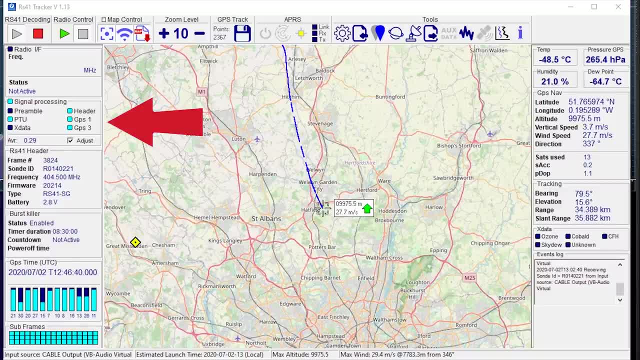 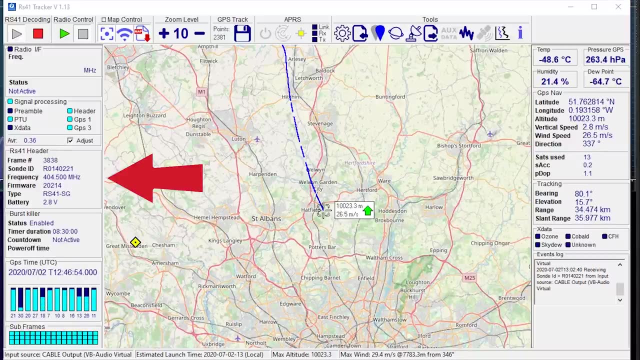 indication. This is useful to see and confirm that our received signal is being decoded by RS-41 tracker. You will also notice that there are indications for the type of data that has been processed, such as the header information or the GPS signal. Now, underneath this, we have the header. 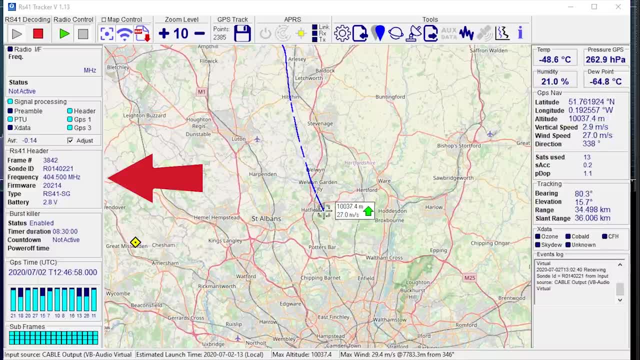 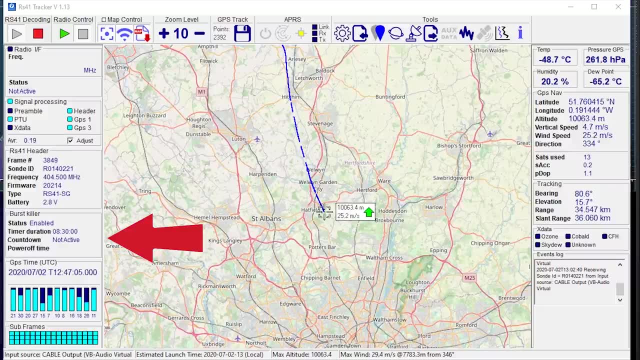 information, which contains the current received frame number, sonde ID and type of sonde and the data Underneath the header information. we have the burst killer status, which is a useful feature to turn off the electronics if a balloon burst is detected. This can be disabled or enabled before. 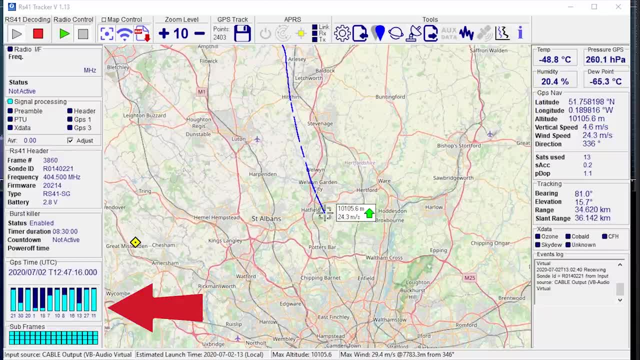 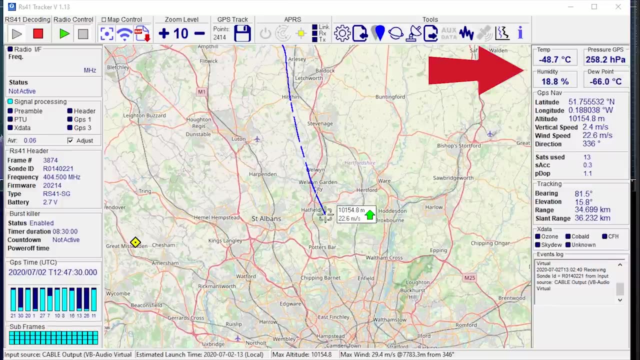 launch Now. lastly, on the left down the bottom, we have the GPS information. This shows the GPS time and a visual indication of how many satellites are being used for the GPS data. Now, as we move over to the top right, we have the sensor information showing temperature, pressure, humidity and dew point. 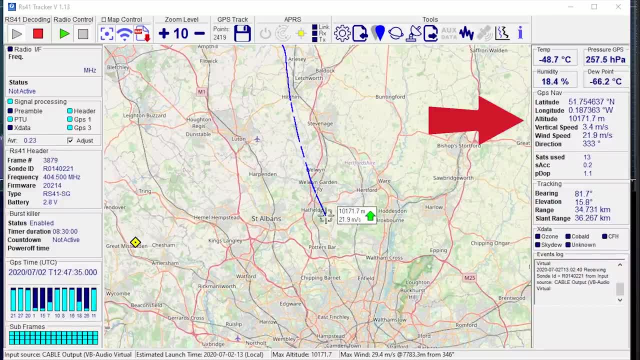 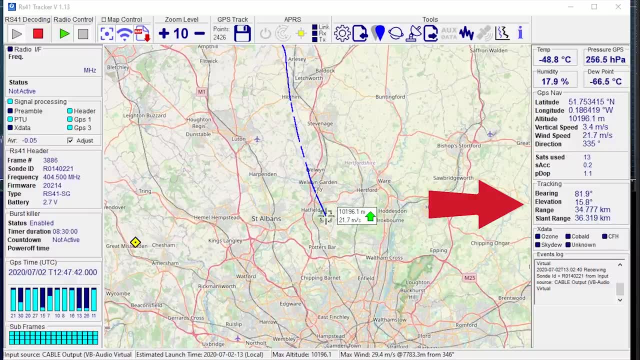 Underneath this we have the GPS navigation data, which is used to display the balloon's location on the map. in the middle, Lower down, we have the tracking information, which is worked out from the latitude and longitude data that we entered into settings earlier, And then, in the middle, we have 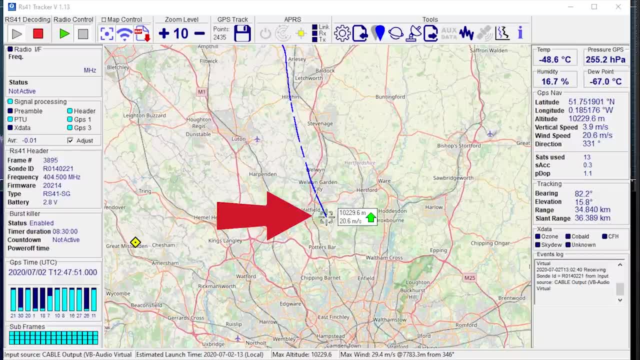 the map. As the balloon is moving you'll notice a small blue trail so you can see where the balloon has been. On the balloon's map marker you'll also notice its current altitude in meters with a little arrow. This balloon was still climbing in altitude. 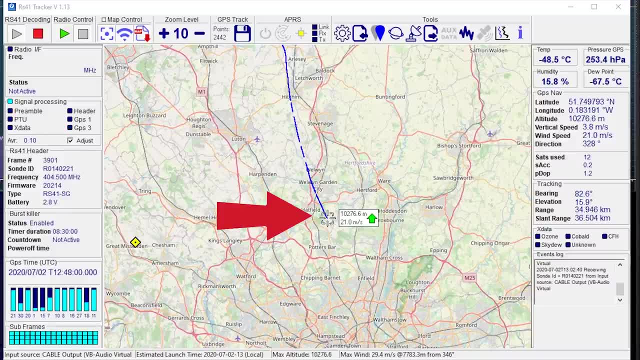 So it's green and pointing up. Now, once the balloon bursts, the little arrow will turn red and will point downwards to indicate that the balloon is falling back to Earth. So here we've, jumped forward to a balloon which is descending. but I wanted to show you a rather 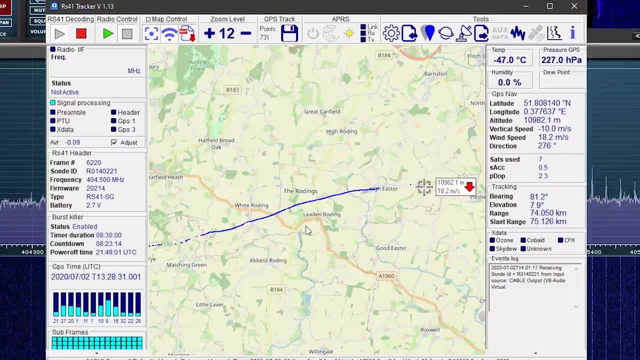 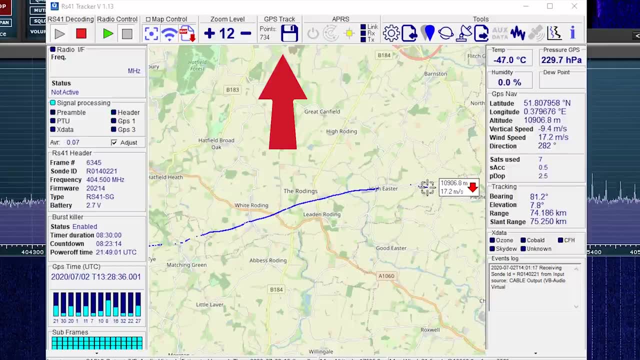 cool feature with Google Earth. So at the top of the menu bar on RS-41 tracker there's an icon button which, when clicked, will export all of the flight recorded. location points to a KML file. You can then load this KML file into Google Earth to see a nice visual representation of the balloon's. 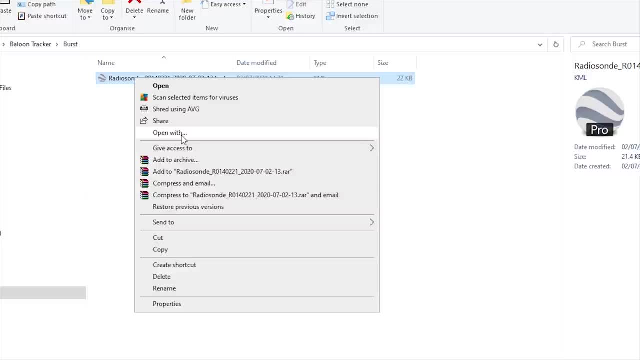 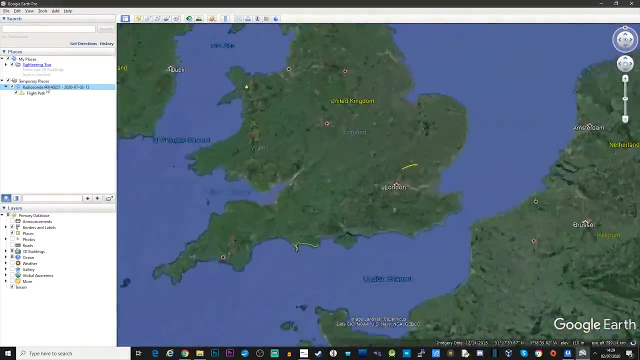 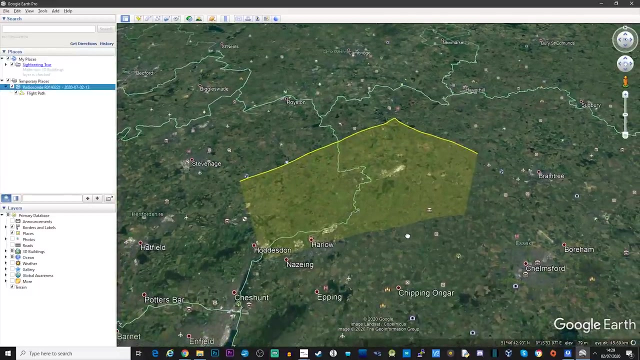 flight. As you can see here, once the KML file has been opened in Google Earth, we will zoom down to its location and we'll be able to view the flight in 3D. Now, using the mouse on my computer, I can move around while zooming in and out. This particular recording was not that long, as I caught the tail.